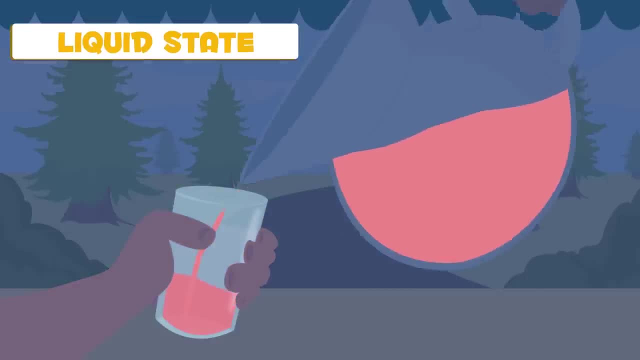 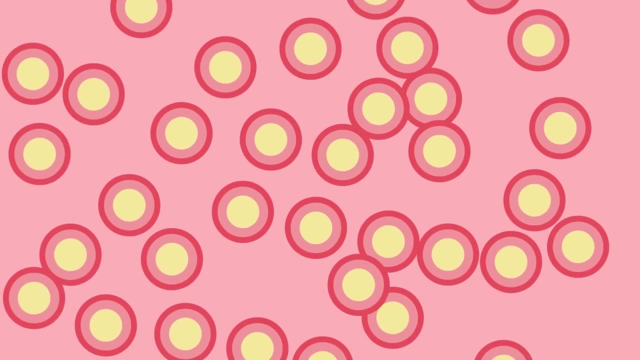 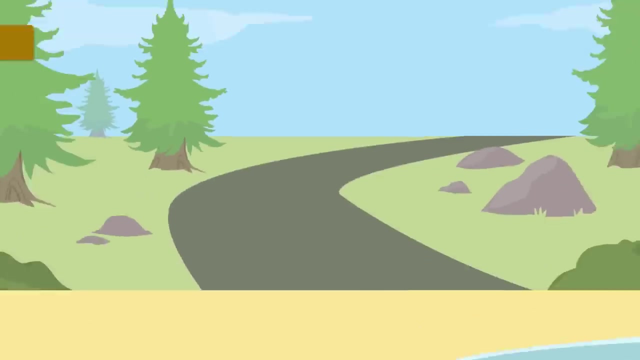 Matter in its liquid state takes on the shape of the container and its volume always stays the same. Particles are separated and condensed. They move freely. Can you see how they're moving? They look like they're dancing. The popsicles we eat are solid. 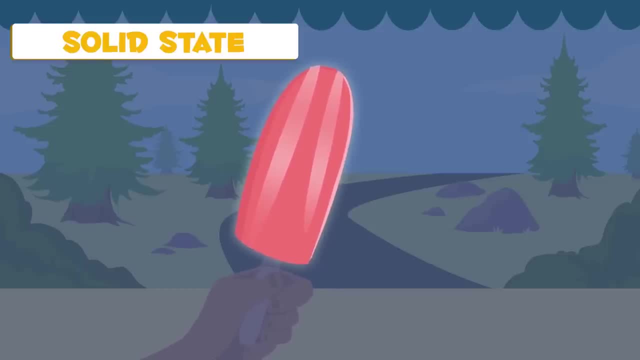 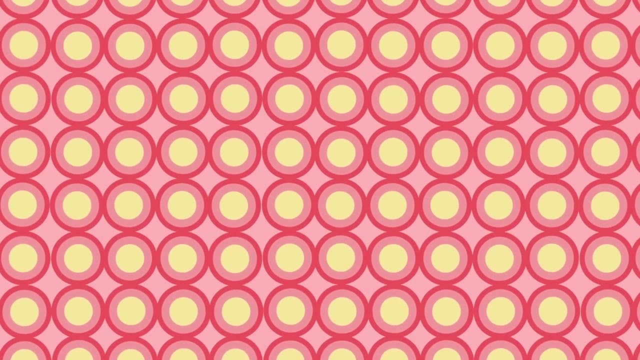 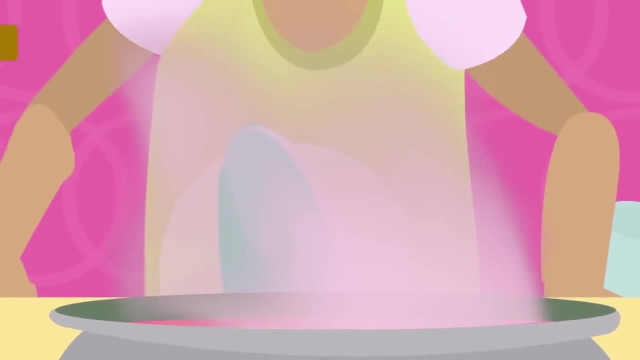 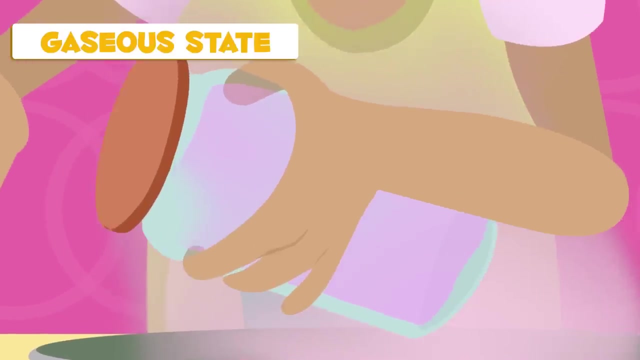 Matter in its solid state is characterized by having a fixed shape and volume. Particles are held together in an organized structure, See, Lastly, the gaseous state. The vapor coming out of the pot is a gas. Matter in its gaseous state can change its volume and shape, taking up the space of its container. 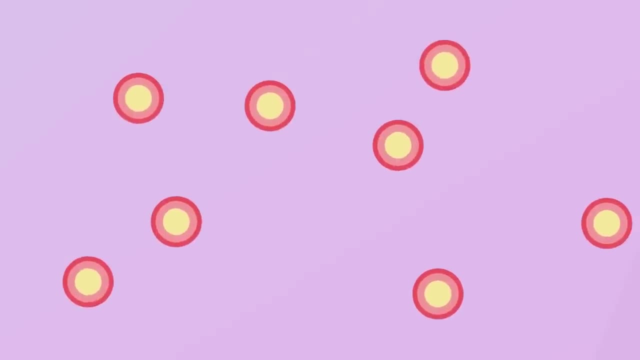 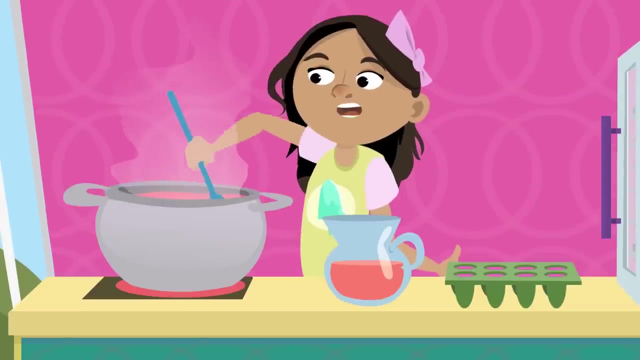 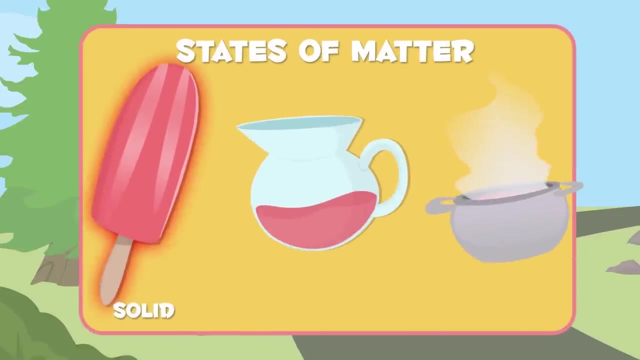 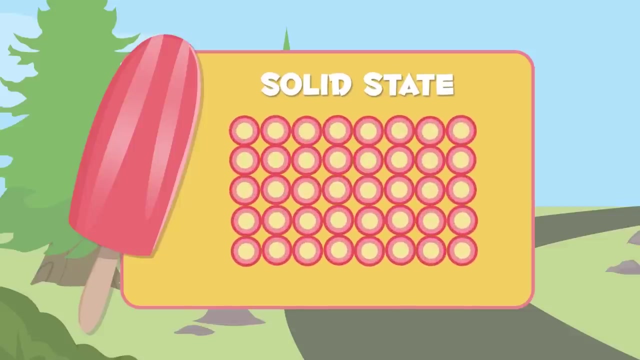 See, Particles are well separated and can move freely. Look, They move like crazy. Did you get the idea? Let's recap a little. Matter exists in three states: Solid, liquid and gas. Solid matter has a definite shape and volume. 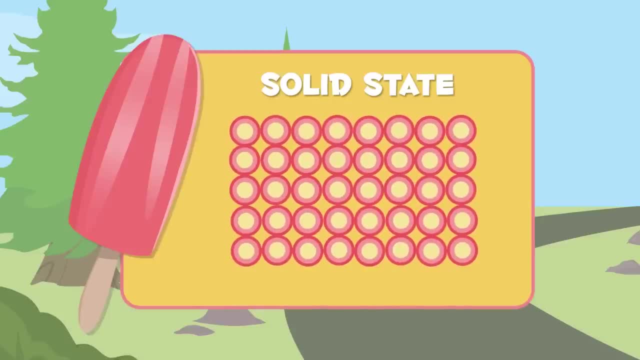 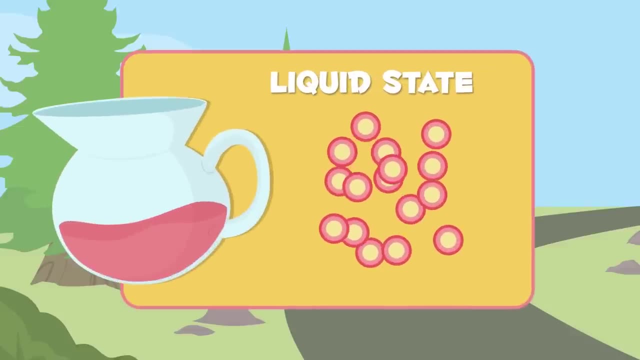 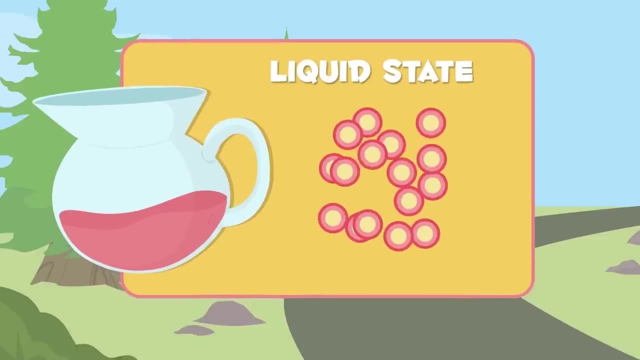 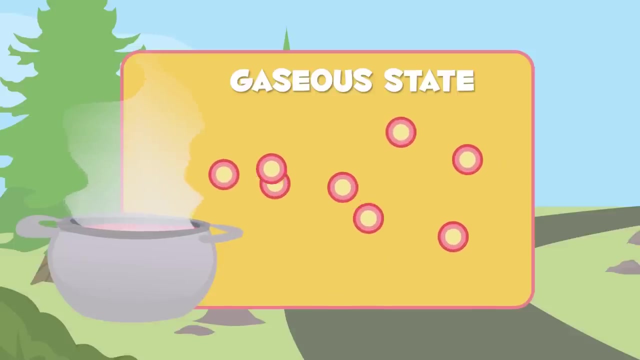 Particles are well organized and held closely together. Liquid matter takes on the shape of its container, occupying always the same space. Besides, particles are separated and can move freely. Gas matter doesn't have a fixed shape or volume. Its particles are well separated and can move freely. 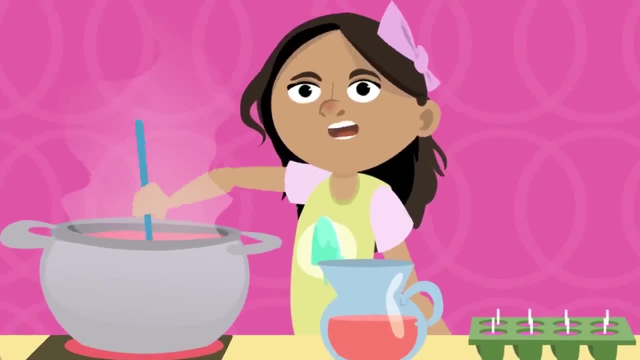 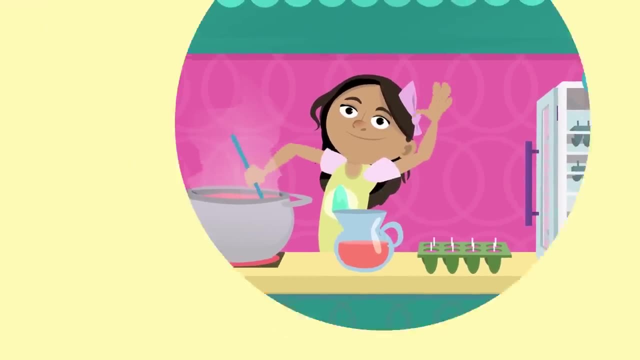 That is all about states of matter. Very interesting, isn't it? Well, I'm leaving now. I won't sell any popsicles if I don't See you around. That's it Perfect. They'll be ready in no time. 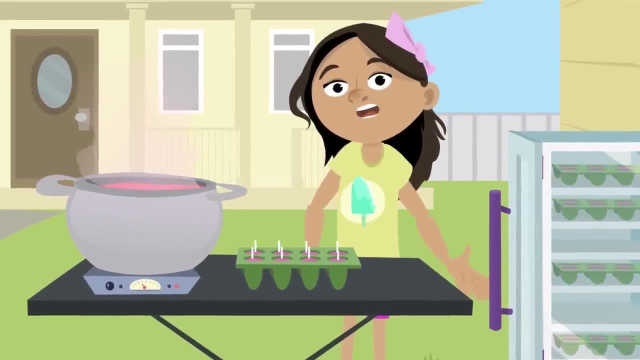 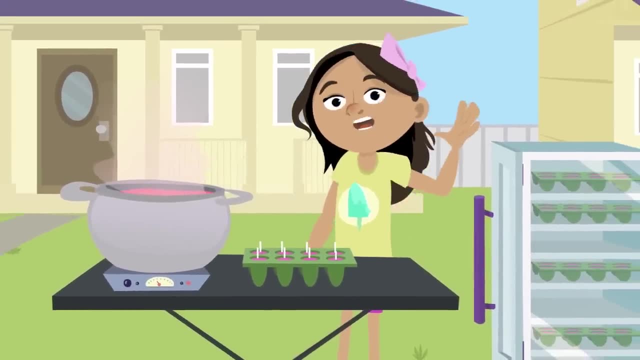 Hey there, I'm making some more popsicles to sell. They taste so good I'm sure they'll sell really fast. These are ready. See, They've become solid because I've put them in the freezer. Have you ever heard of the word solidification? 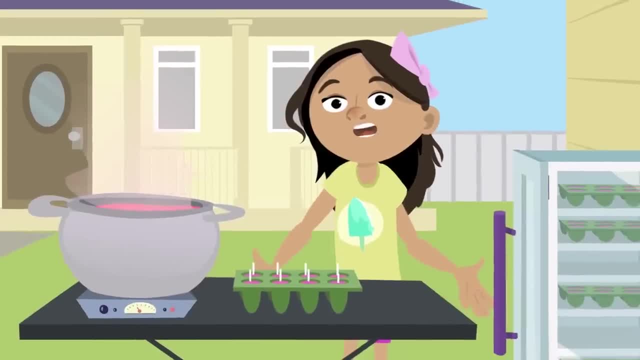 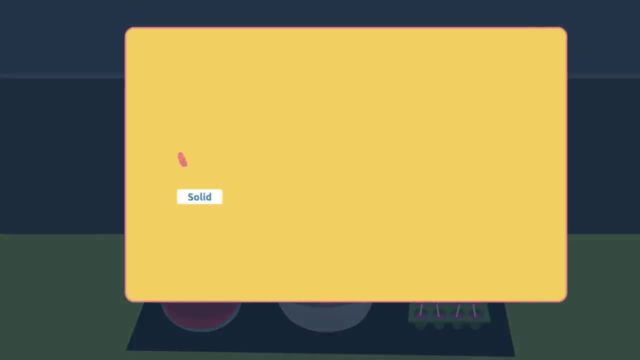 It's one of the changes in states of matter. There are more changes, don't worry. I'll explain all about them. You already know that matter exists in three states: Solid, liquid and gas. A change in state happens when we heat or cool matter. 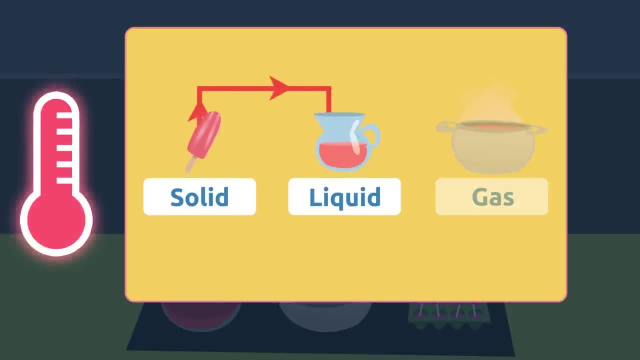 If we heat solid matter, it becomes a liquid. We call this process fusion. If we heat liquid matter, it becomes a gas. We call this process vaporization. These two processes can occur the other way around. This happens when we cool matter instead of applying heat. 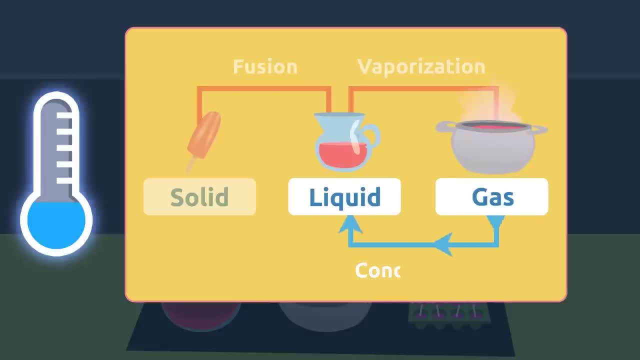 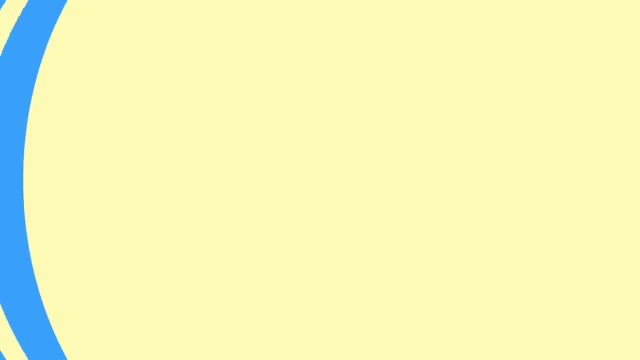 If we cool a gas, it becomes a liquid. This process is called fusion. This process is called condensation. If we freeze liquid matter, it will become a solid. This process is called solidification. Oh no, the popsicles have melted. 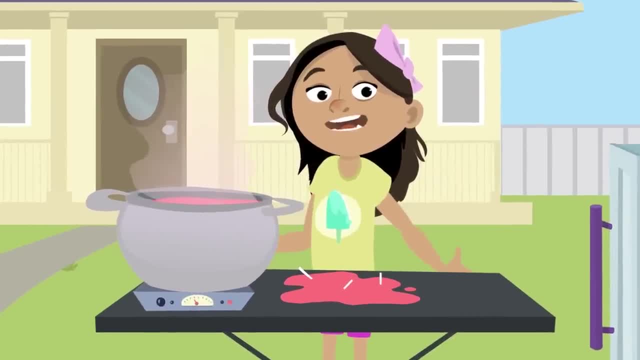 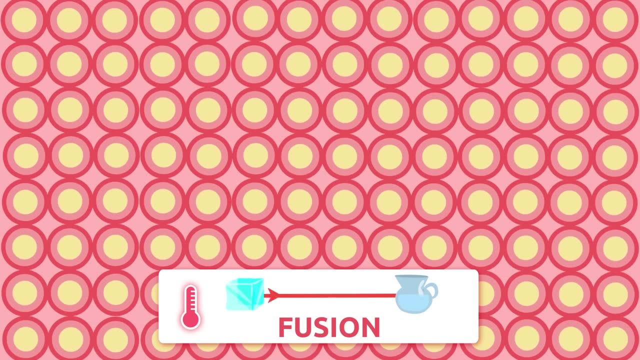 I completely forgot about them. Do you remember how we call the change from solid to liquid Fusion? When a solid becomes a liquid, it's called fusion. When the temperature of a solid rises, the particles that make up matter start detaching from one another. 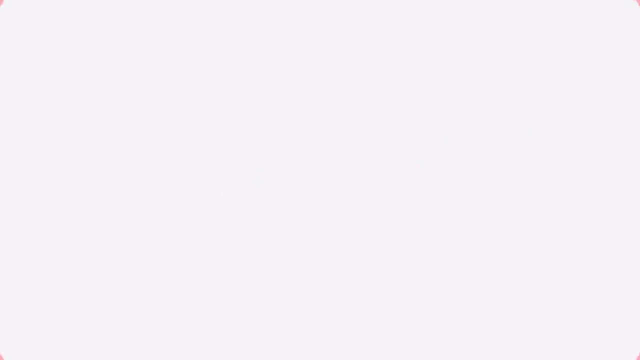 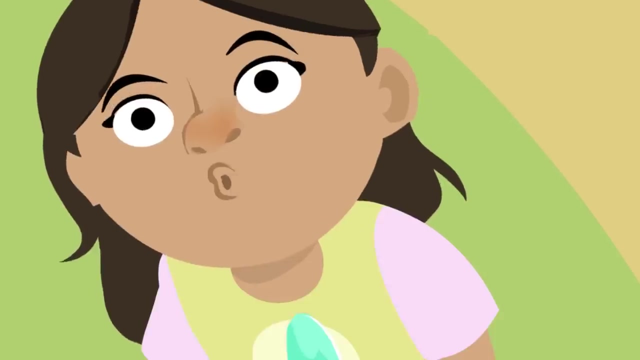 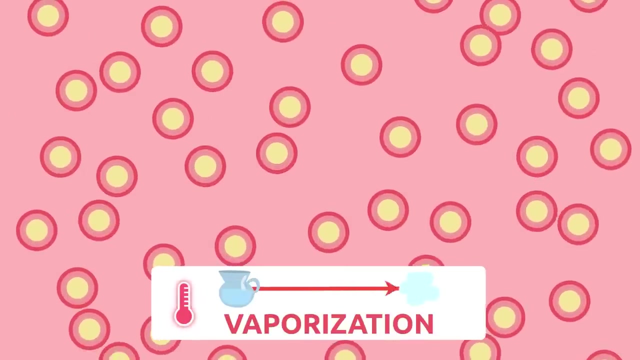 and move more freely. See: Liquid turns into gas when heated. Do you remember how we call this process? When a liquid becomes gas, it's called vaporization. When a liquid is heated, the bonds among the particles that make up matter become more loose. 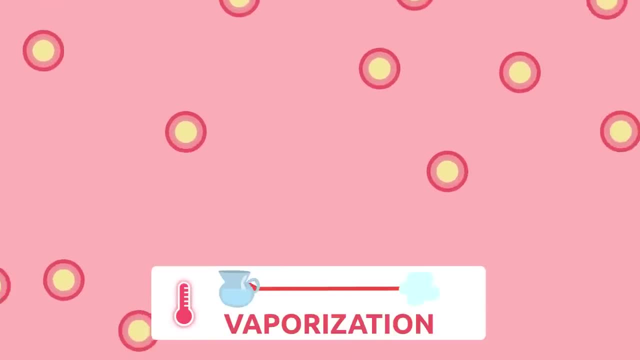 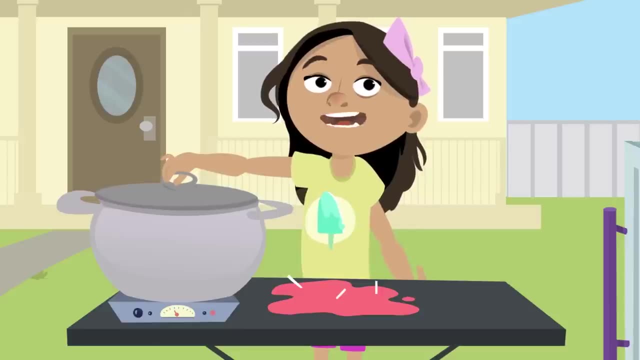 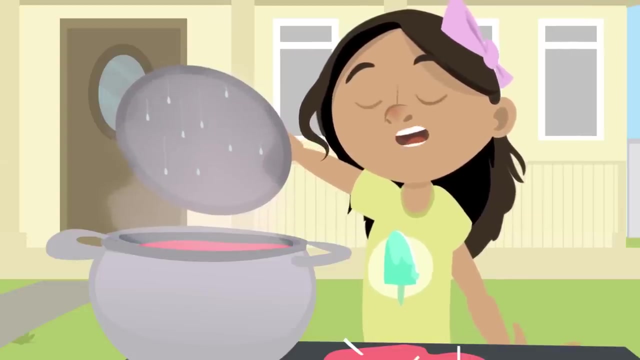 so particles move around freely. What if I cover this pot? What do you think might happen? Water vapor cools as it reaches the lid and its state changes from gaseous to liquid. Do you remember how we call this process? I've just told you, haven't I? 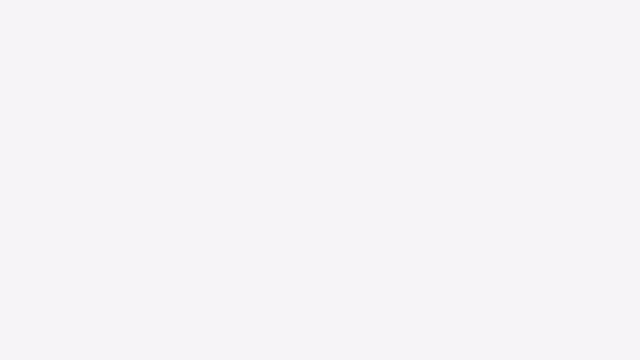 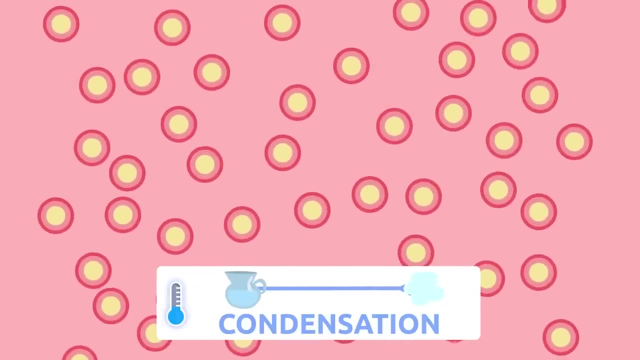 The change from gaseous to liquid is called condensation. As a gas cools, the particles that make up matter start coming closer to one another and move around more slowly. This will continue to happen until matter solidifies completely. I think the popsicles I froze up earlier are just about ready. 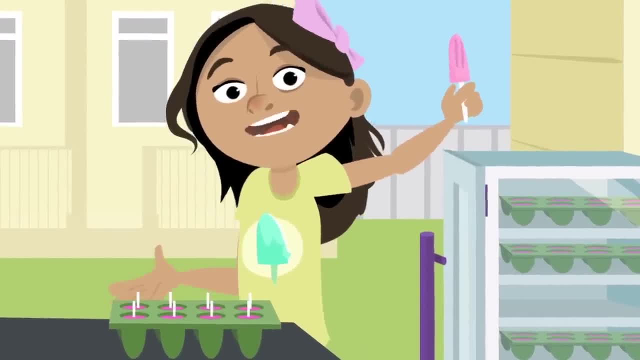 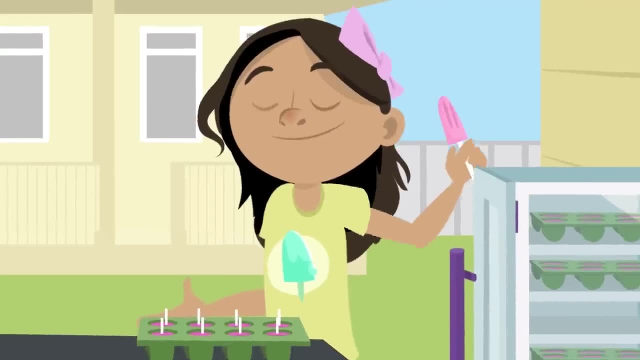 That's right. I put some popsicle molds in the freezer a while ago. The liquid in the molds must have frozen up by now. The change from liquid to solid is called. Come on, you know this. I told you before It's called solidification.